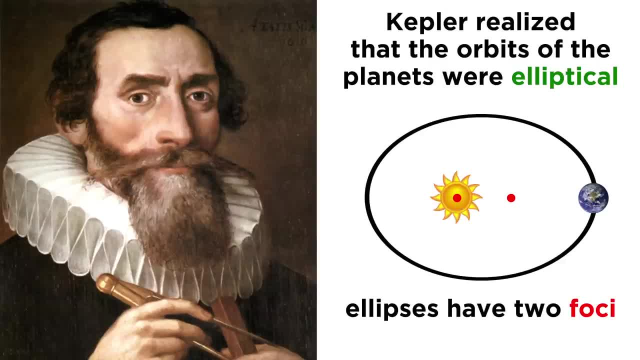 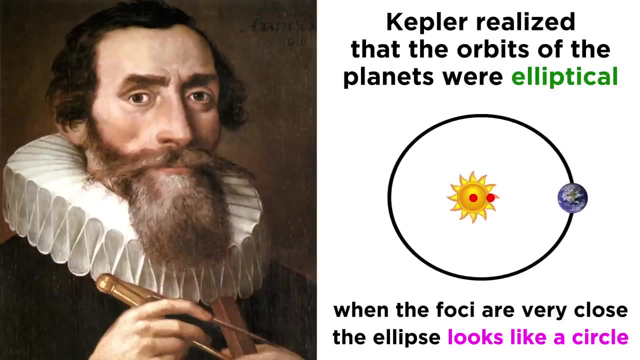 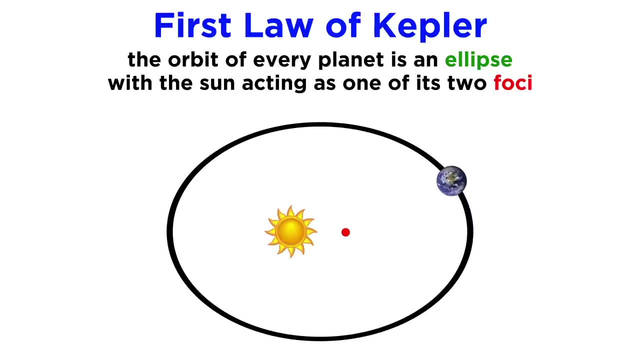 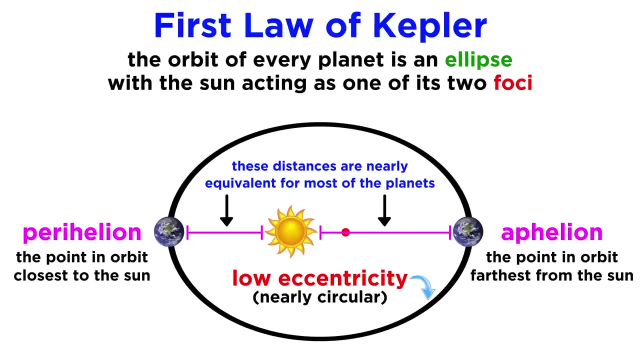 I hope you enjoyed this video and I'll see you in the next one. Bye, They are not circles, They are ellipses. This fact is the first of three laws, known as Kepler's laws, which essentially marked the birth of celestial mechanics. 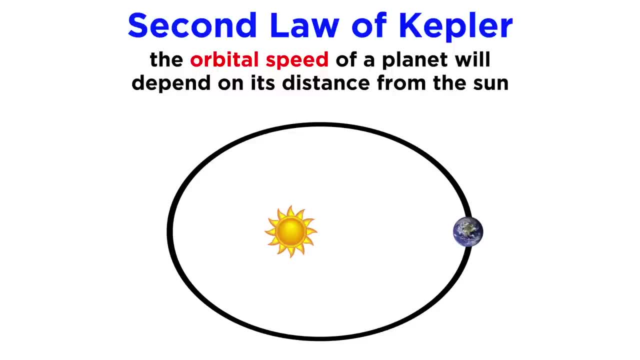 The second of Kepler's laws says that the orbital speed of a planet will vary according to its distance from the sun. it slows down when further away and speeds up when closer in. A little more formally, it says that a planet will sweep out equal areas over equal time. 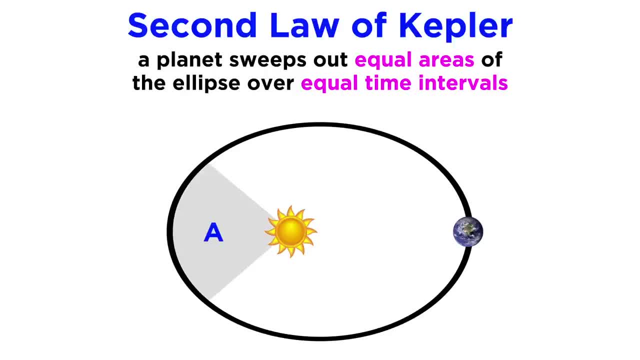 intervals. So if we take this area A of the ellipse involving a part of the orbit that is closer to the sun and this other equal area A of the ellipse involving a part of the orbit that is further away from the sun, the distances travelled by the planet either C to D or 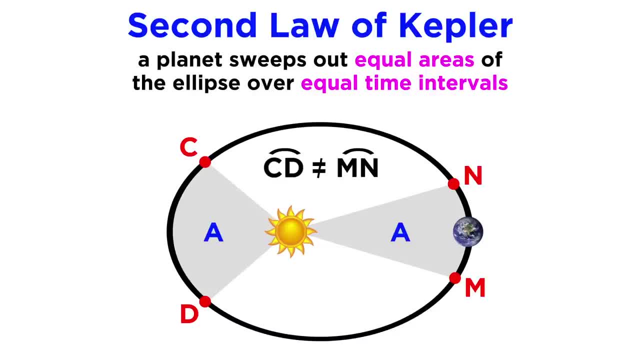 M to N in order to sweep out. these areas are of different dimensions. This is called the Kepler's law. However, the planet moves faster when close and slower when far away, in a manner that results in precisely equivalent time intervals. 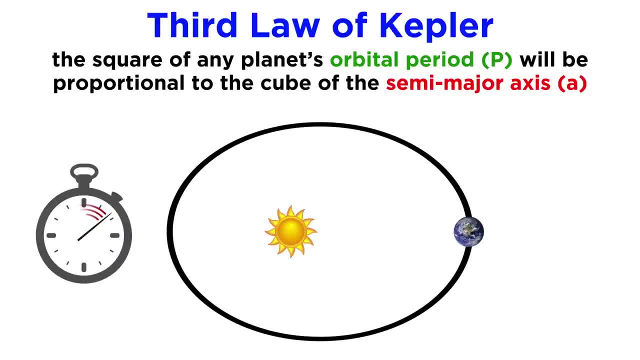 And Kepler's third law states that the amount of time a planet takes to orbit the sun or its period is related to the length of the semi-major axis, That's this length here, or half the major axis, which is the longer axis of the ellipse. 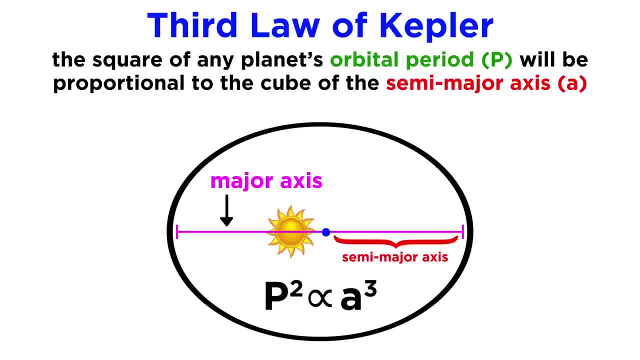 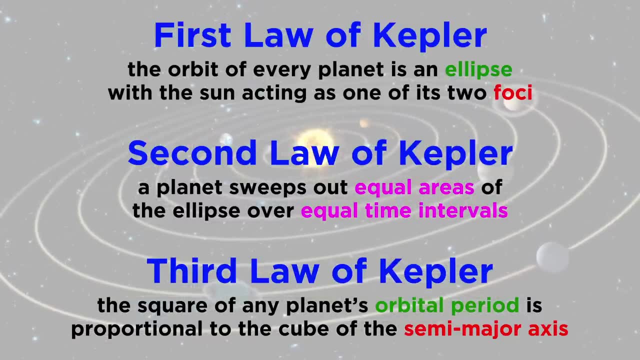 Specifically, P squared is proportional to A cubed when measured in years and astronomical units, and the precise relationship will depend on the mass of the planet. These laws are derived from observation, and when we use these laws to predict the positions of the planets at any future moment, we find that they are extraordinary. 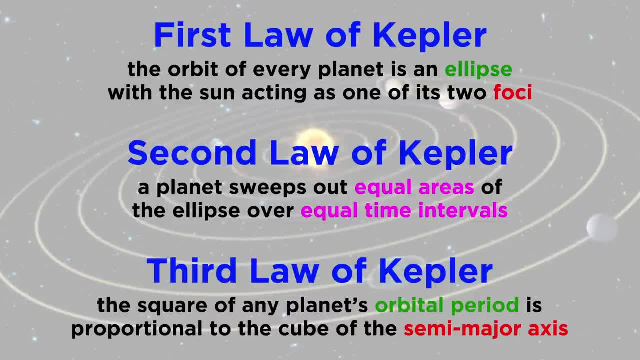 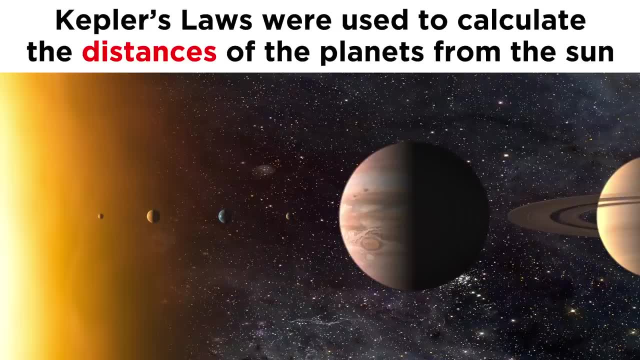 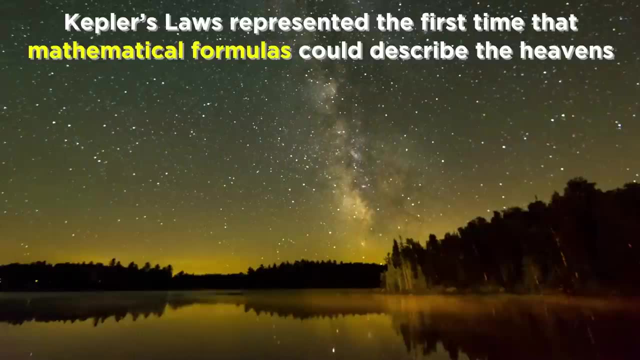 Extremely precise, which is all that any good science can hope to do. These laws were used to calculate the relative distances of all the planets from the sun and had other practical applications as well, but the impact of these laws was much deeper than the merely practical. 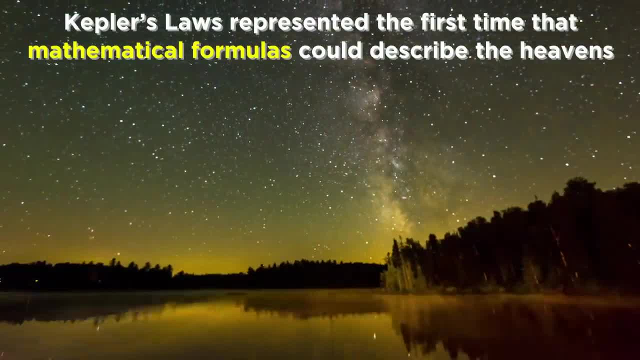 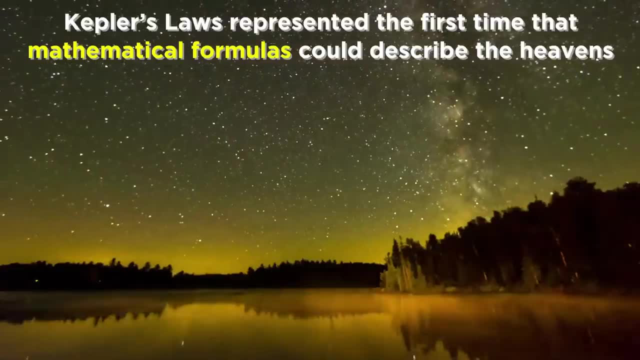 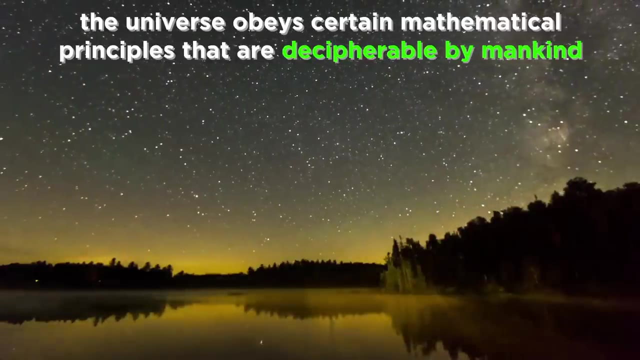 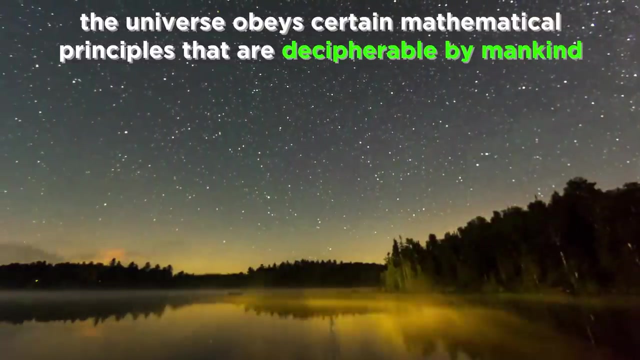 These laws represented the first time that a handful of extremely simple mathematical formulas were able to describe and predict the motions of the heavens to the utmost precision. It was undeniable proof that the universe obeys mathematical principles that are decipherable by mankind, which is the basis of the revolution that produced modern scientific thought. 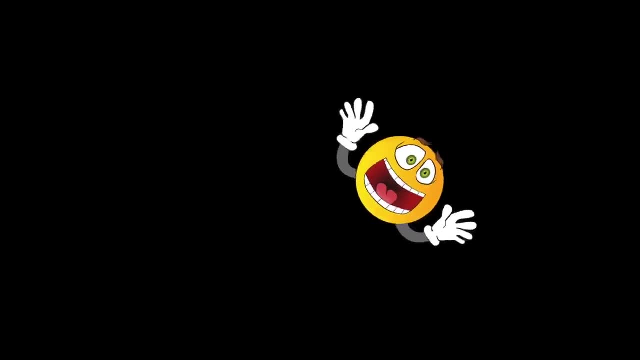 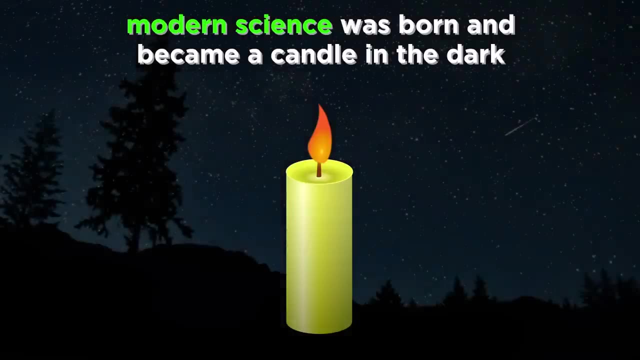 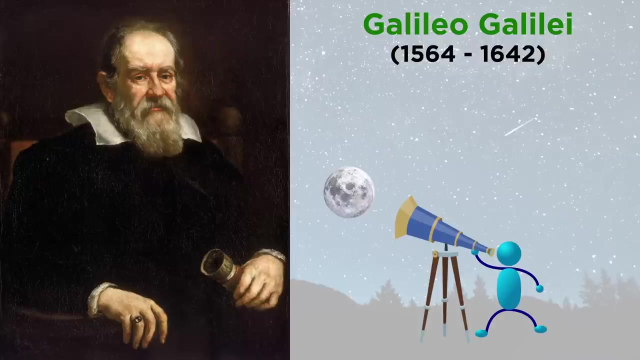 We were no longer helpless victims of the natural world tumbling in darkness. We ignited a spark that lit the candle, that shined a light such that we began to understand our surroundings. An Italian scientist, Galileo Galilei, was observing the same night sky, but focusing 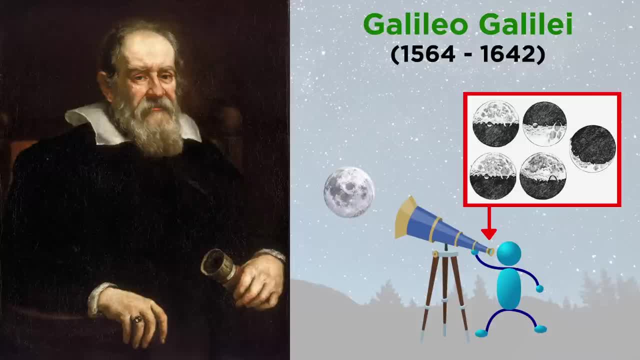 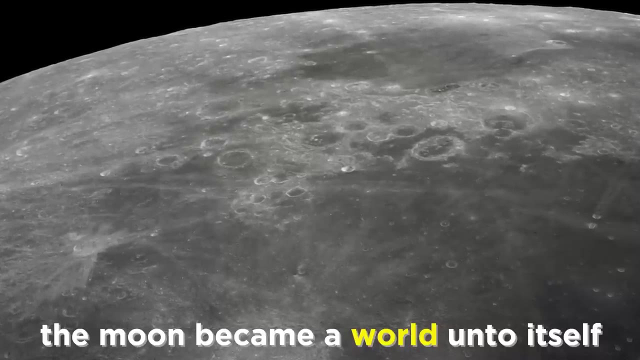 on entirely different observations. He used the best telescopes of the time to see that the moon had distinct terrestrial features, like mountains and craters, just like the earth. This transformed the moon into a world unto itself, rather than just a mysterious glowing. 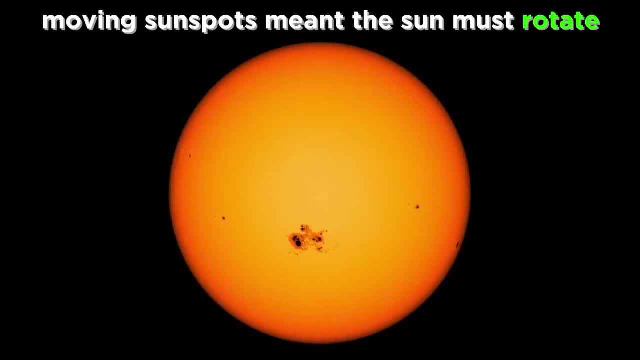 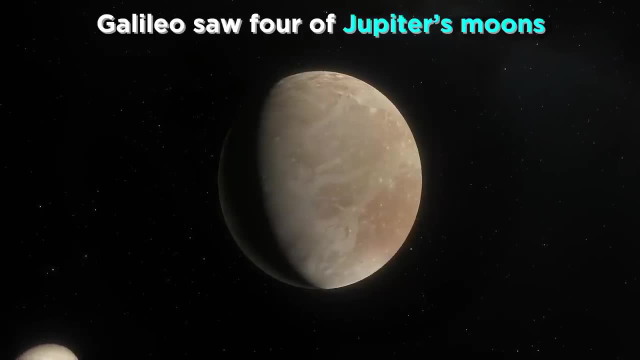 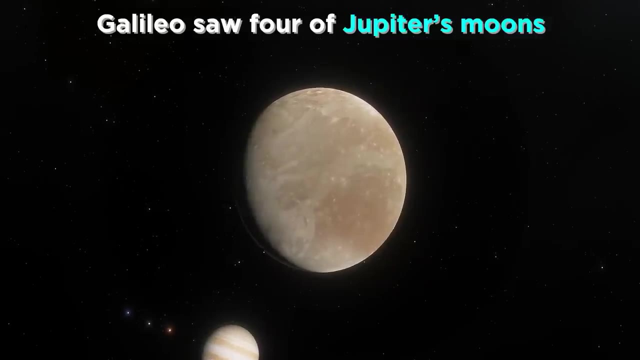 disk. He noticed the dark sunspots on the sun, which changed position over time, thereby deducing the rotation of the sun. He observed Jupiter's moons and as they orbit Jupiter. this proved that not everything in the solar system orbits around the sun or the earth, no matter which of the two. you 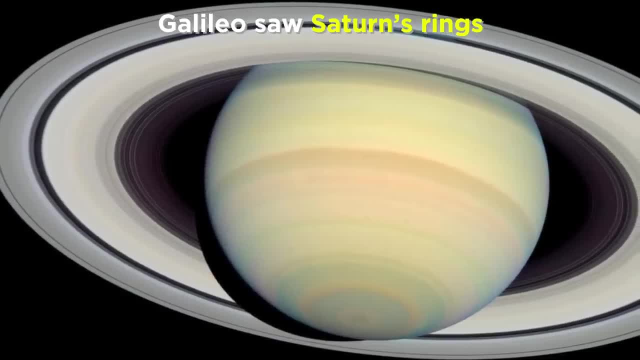 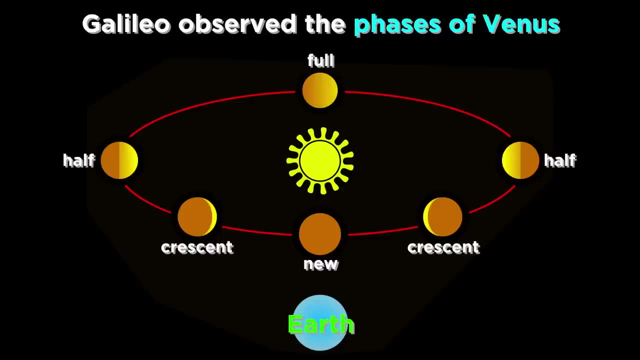 put at the center. He saw what we would later understand to be Saturn's rings. He observed the phases of Venus, demonstrating that it must be in orbit around the sun Just as the moon is in orbit around the earth. the final nail in the coffin for the geocentric 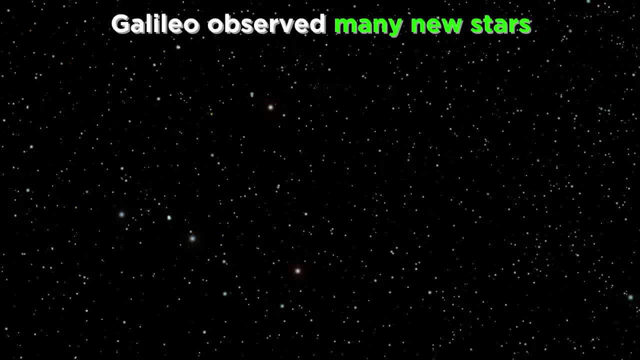 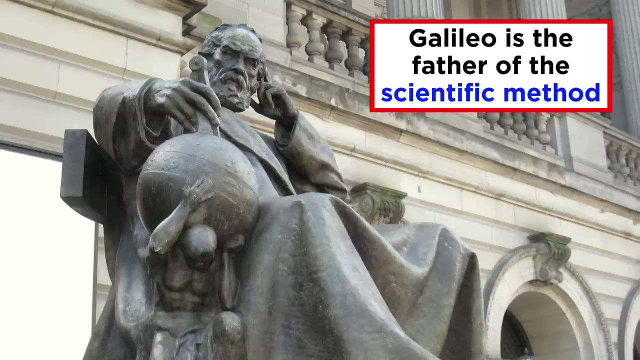 model, And he observed far more stars than were previously visible to the naked eye, indicating that the universe is much bigger than was thought at the time. Although he is often better remembered for being the father of the scientific method, as well as all of his contributions to classical mechanics, Galileo did as much as anyone else. 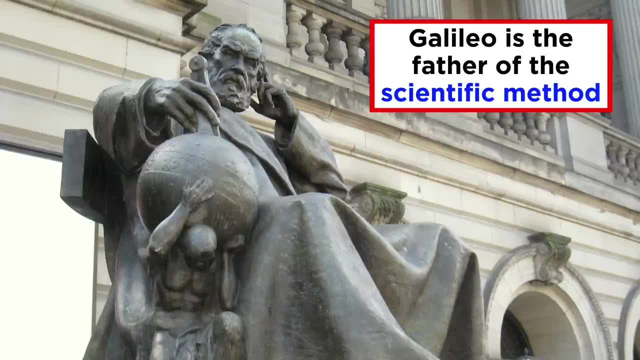 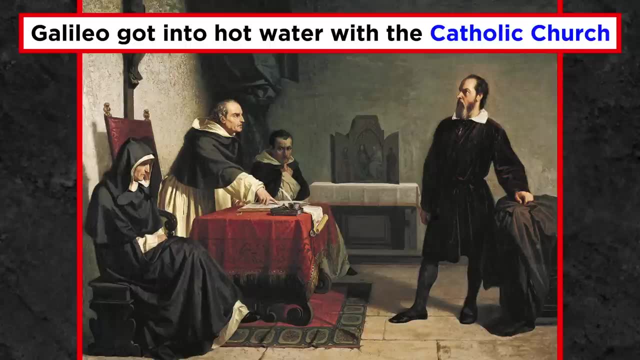 ever did to rewrite our perception of the cosmos. This earned him the same contentious status with the Catholic Church as Giordano Bruno, but Galileo was a little less stubborn, recanting his work under pressure, and he was sentenced only to house arrest, living the last of his years confined to his home. 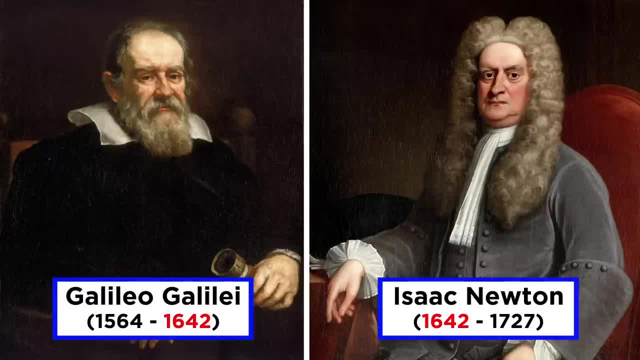 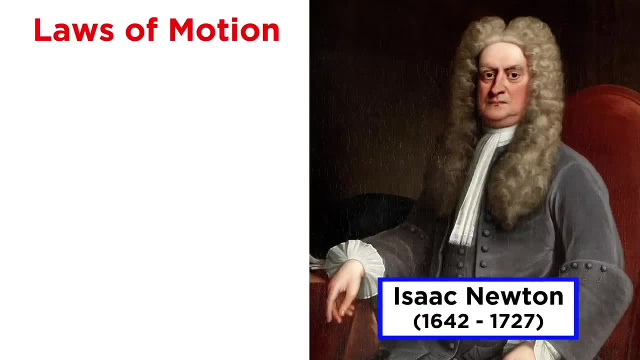 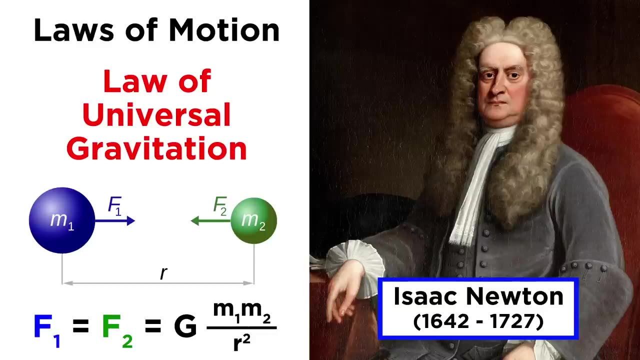 The year that Galileo died was the same year that Sir Isaac Newton was born, and his contributions to science were irreplaceable. Beyond his laws of motion, he also provided the first accurate description of the gravitational force, which was then used, in a stroke of genius, to demonstrate that objects fall to. 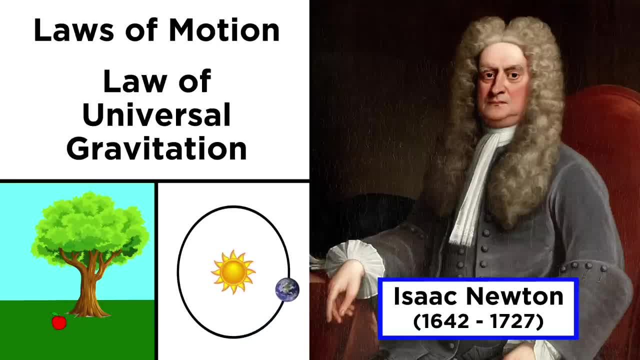 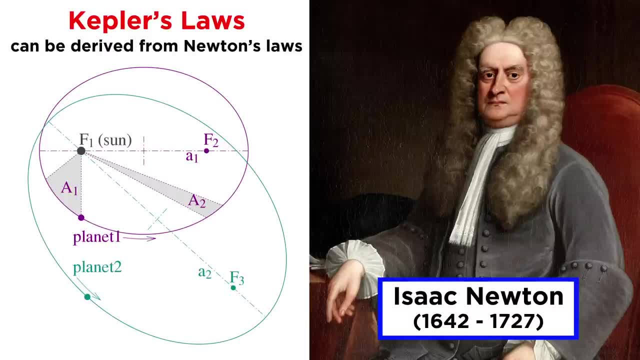 the earth for the same reason that the earth goes around the sun, and he thereby demonstrated that all three of Kepler's laws were consequences of his own laws of motion and universal gravitation. All of this is described in detail in my classical fiction book, The Law of Motion. 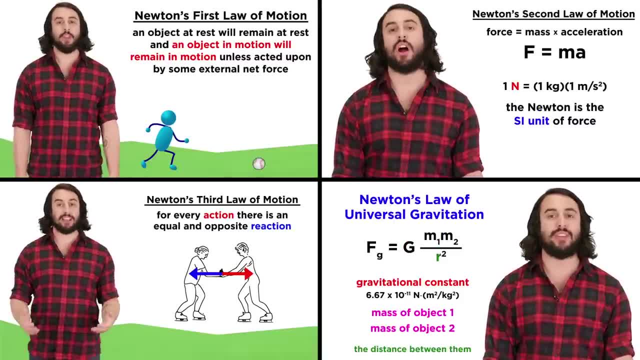 I hope you enjoyed it. If you did, I'd love to hear what you thought of it. and if you did, I'd love to hear what you thought of it. If you did, I'd love to hear what you thought of it. 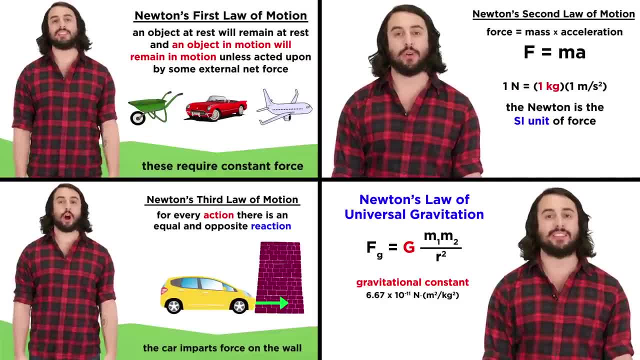 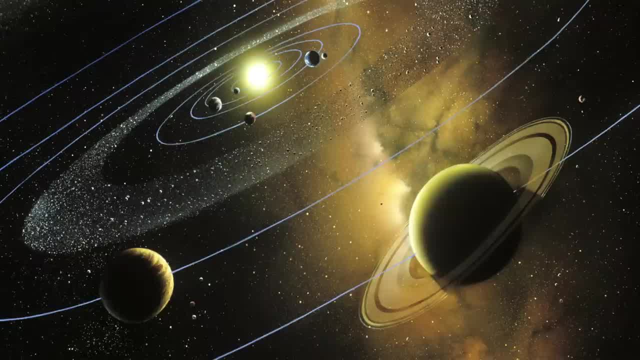 So head there for more information if you're interested. Otherwise, let's continue our story. From Ptolemy to Newton, our picture of the solar system changed dramatically, leaving us with a perception about the universe that did not change much until the twentieth century. 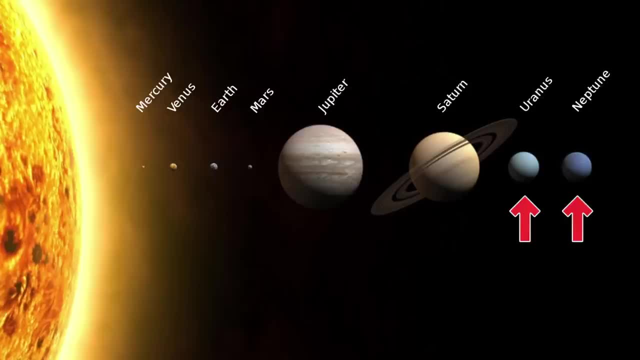 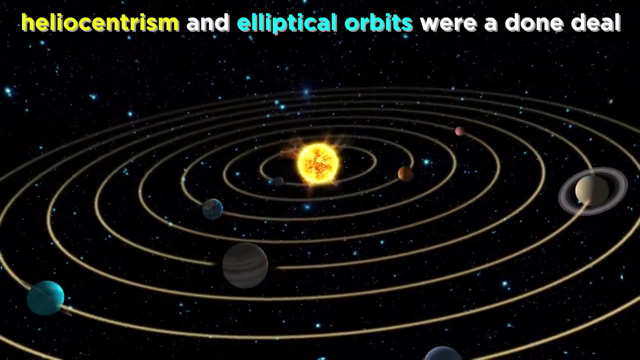 We discovered two more planets beyond Saturn, as well as a host of other small objects, but heliocentrism and the elliptical paths of the planets around the sun were locked in, With some historical perspective taken care of. let's move forward and take a closer.